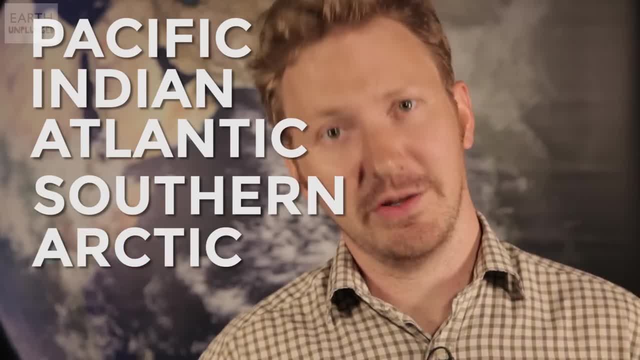 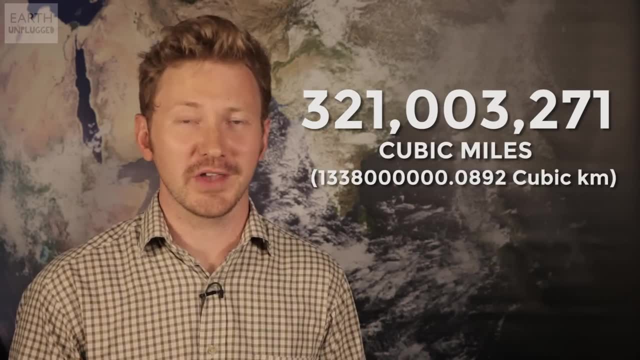 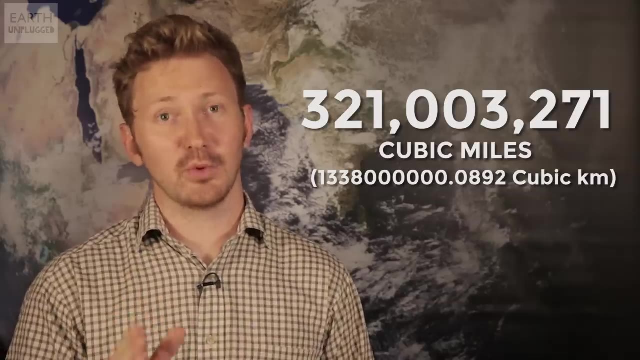 the Indian, the Atlantic, the Southern and the Arctic Ocean. that's the cold one. Now, within all that water, around 321,003,271 cubic miles, there exists a plethora of creatures, but one that can barely be seen by the naked eye is arguably the most important of all. 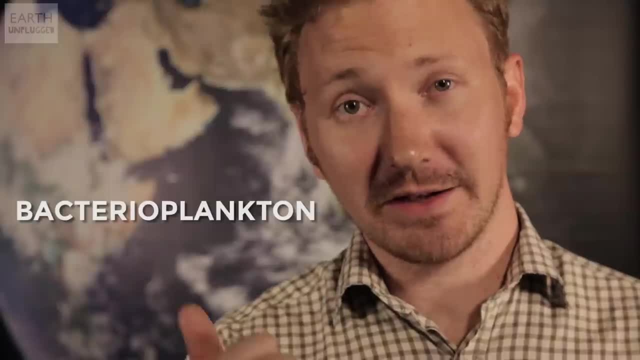 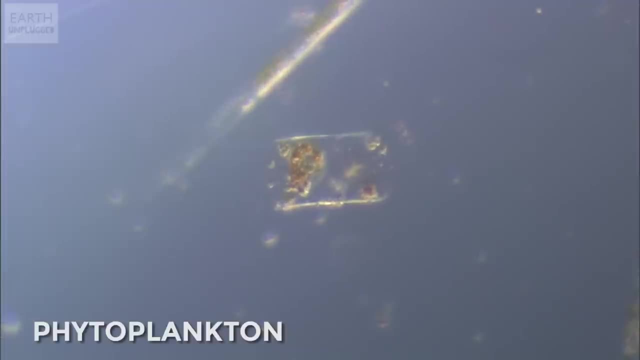 Plankton. There are three main groups of these organisms. There's Bacterioplankton, made up of bacteria and archaea, that's single-celled microorganisms. There's Phytoplankton, which is plant-based, And finally, Zooplankton, which are predominantly tiny living animals. 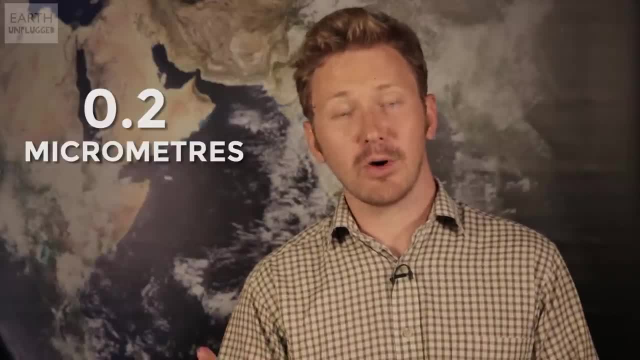 They can be as small as 0.2 micrometres, a micrometre being a thousandth of a millimetre, that's smaller than the diameter of a human hair. Now, while plankton may appear to be very small, they can also be very small. 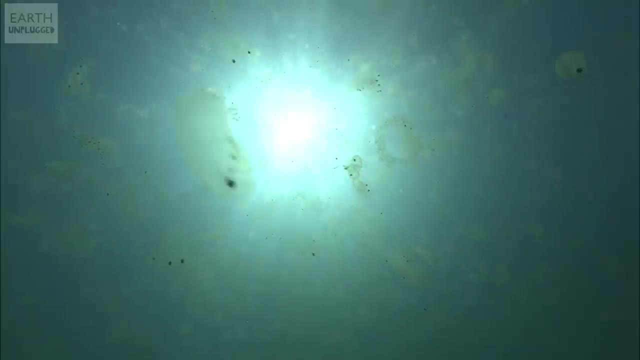 Now, while plankton may appear to be very small, they can also be very small. They appear to be aimless drifters, directionless in their movement. In life, they play a key role and are perhaps the most vital organism on earth. 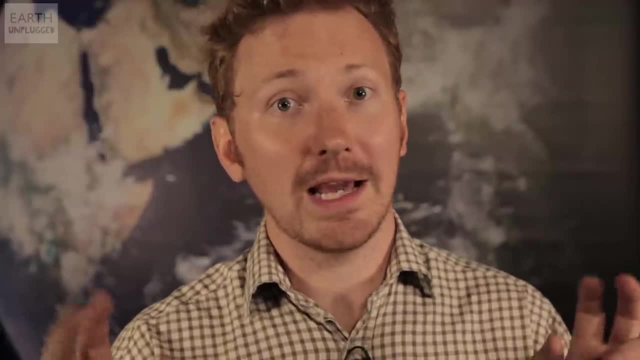 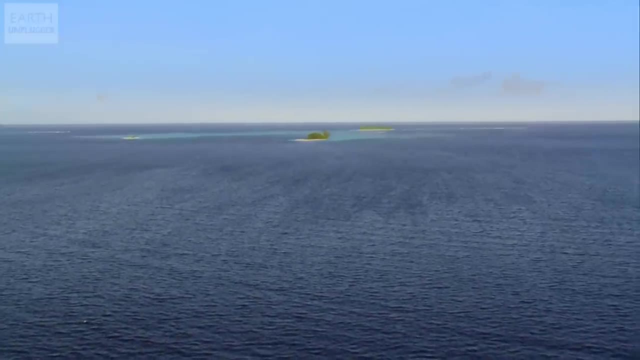 You see, each and every plankton, or to be more precise, plankta, perform a unique job And if they were to suddenly disappear, quite frankly, the ocean, the earth and us would be stuffed. Without them, the whole marine ecosystem would soon collapse, With no phytoplankton to clear. up the waste. the zooplankton have nothing to eat. And with no plankton, what are the small predators going to eat? Oceanic megafauna like dolphins, whales and sharks with nothing to eat would soon perish. Now plankton also account for around 20% of all photosynthesis. 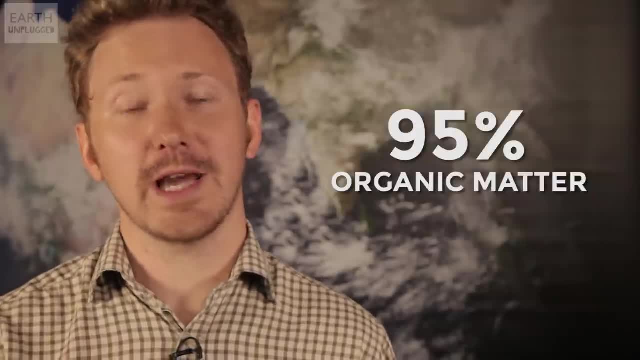 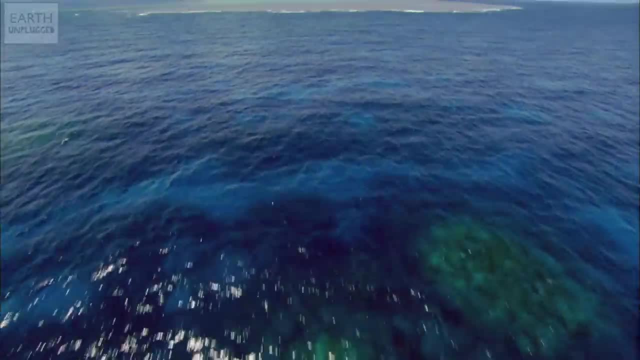 on earth and around 95% of the recycling of organic matter in the ocean. Yep, without plankton, the oceans would be a barren wasteland of watery nothingness. But it doesn't stop in the water. With the foundation of the food chain gone, seabirds with nothing to eat would soon fall from the sky. 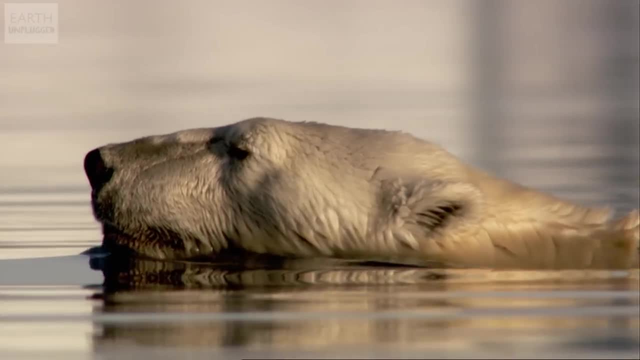 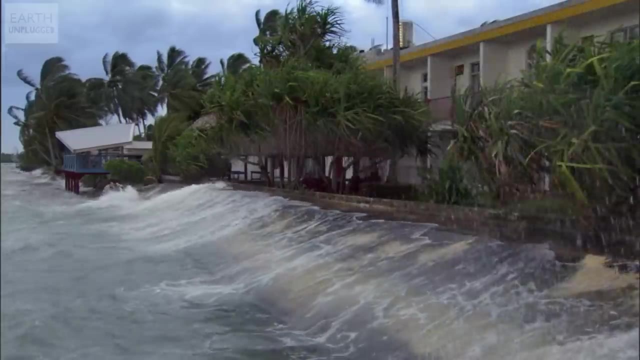 Seals Dead through hunger. Polar bears- Yep, they're goners too, And this is where a world without plankton would start to affect us, With around 70% of the human population living within 60km of the coastline. catching and depending on around 80 million tonnes of fish per year. no plankton means no fish, no local trade and economic collapse. No fish with your chips and ultimately, millions of hungry people Fancy popping out to do the weekly shop in your car. 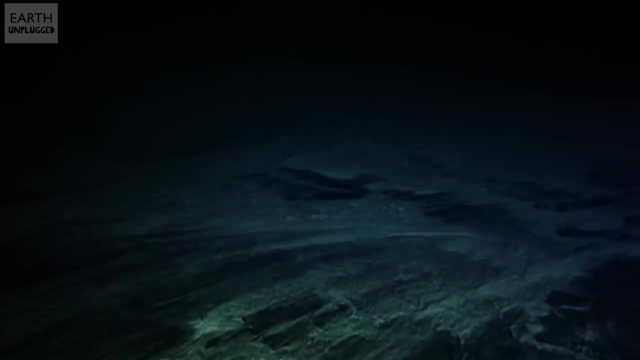 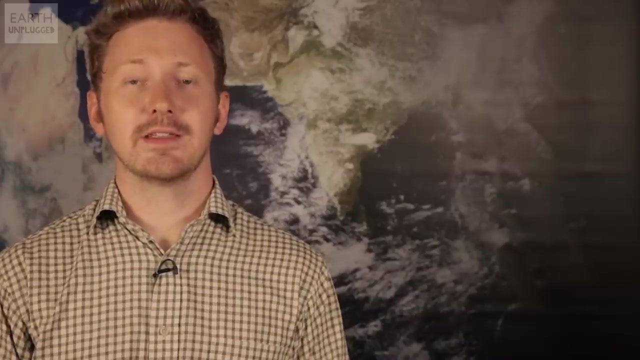 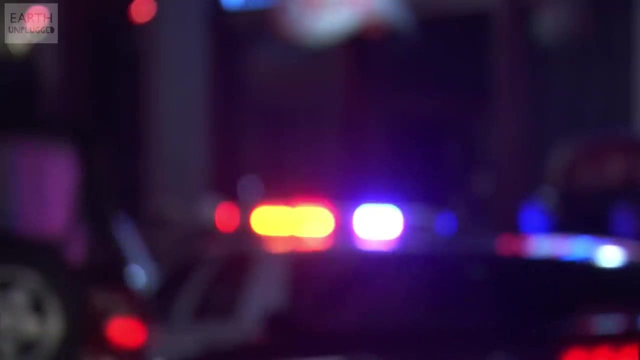 Er? no, You see. some decaying plankton and their fecal pellets drift down to the ocean floor and take with them the carbon they contain. Over millions of years, this matter creates the world's oil and gas reserves. So no plankton, no fuel. So your car won't work, factories would fall silent.